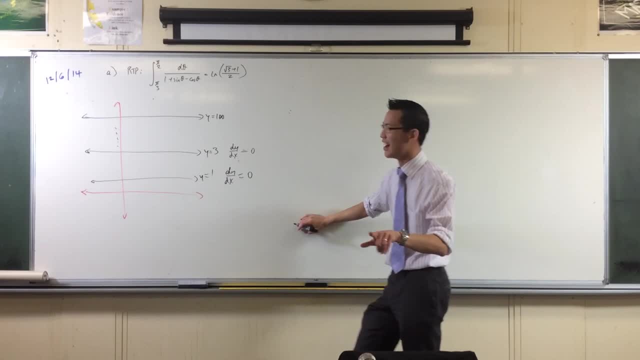 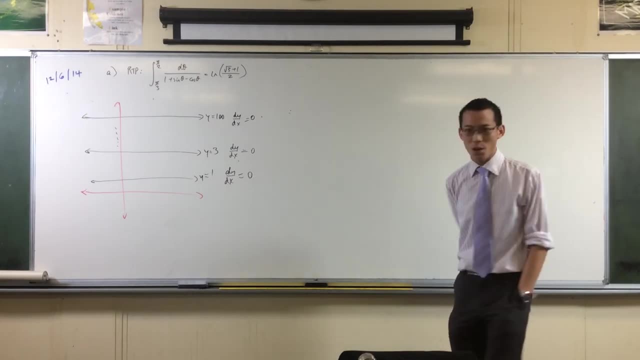 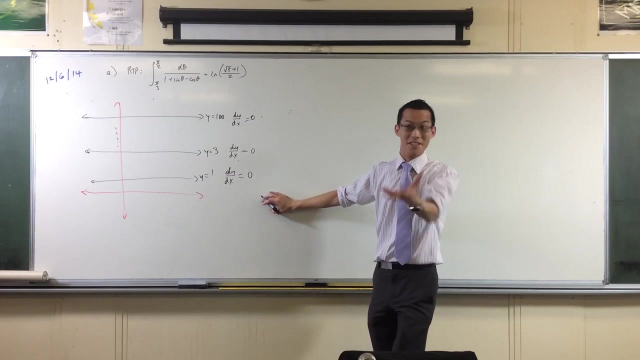 on. The numbers are bigger here, So be careful. okay, I think I think it's 0.. Is that okay? Hmm, So therefore, I conclude, I look at these and these are sophisticated functions, but I'm quite good at maths. I. 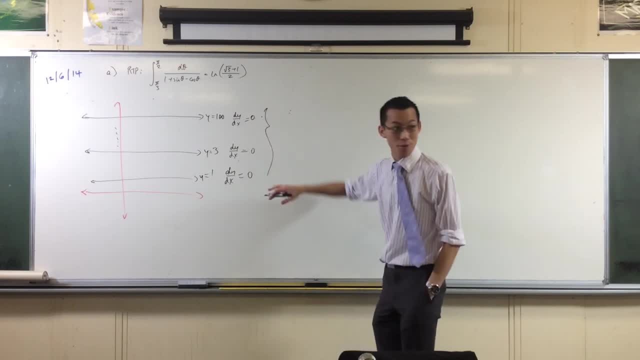 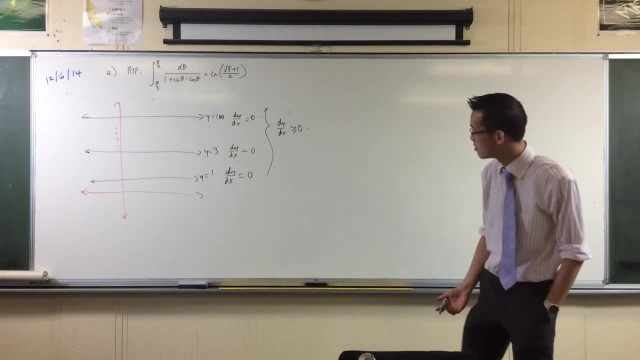 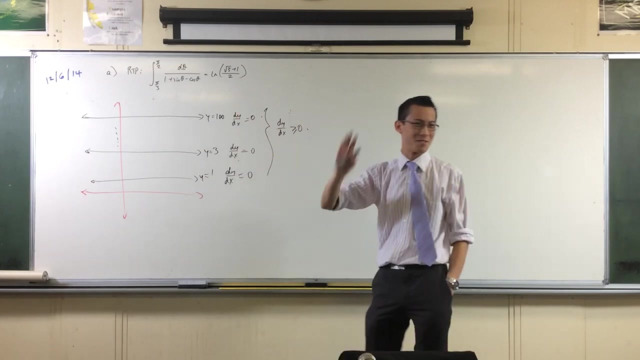 do extension too, right? So I know things like this. I can say for all these three functions that dy and dx is greater than or equal to 0. Isn't it? It is All of these satisfy this right. But you guys all said these weren't increasing functions. What liars. That means they're. 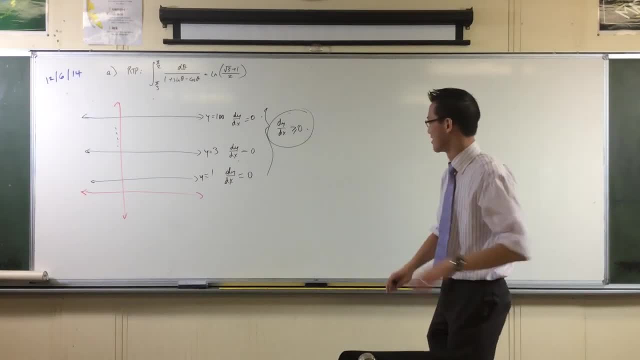 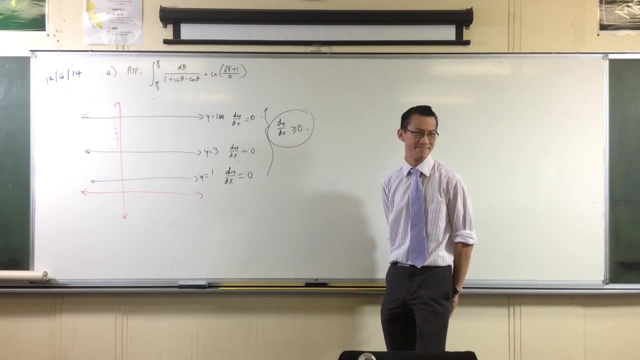 increasing. right, Of course they're increasing. You're all fired. Don't do extension too anymore. You've missed it. Or did I do something wrong? What's wrong? Why? why is my conclusion that these are increasing functions, because this is true of all of them? Why is it wrong? Oh, 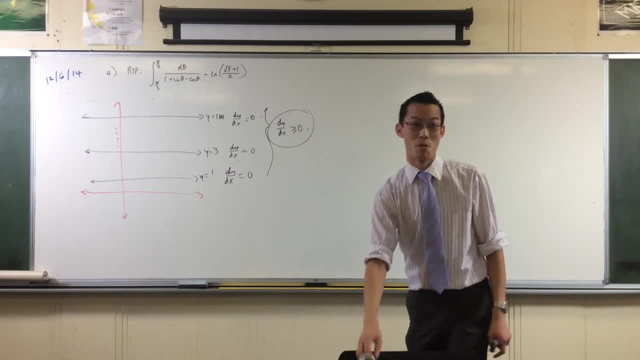 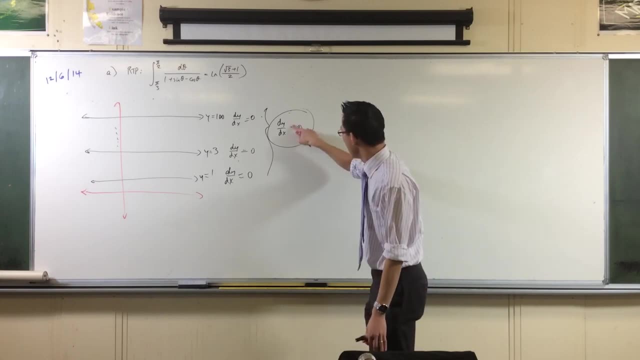 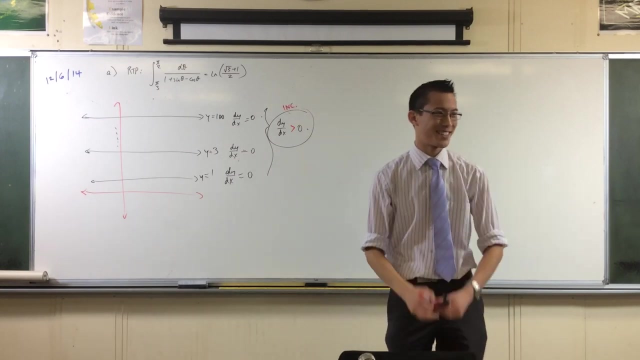 oh, There's a small problem here. Small problem, It's not. it's not greater than or equal to 0. that makes it increasing function. right, It should be greater than 0.. That's an increasing function. Oh, but that's not what you told. 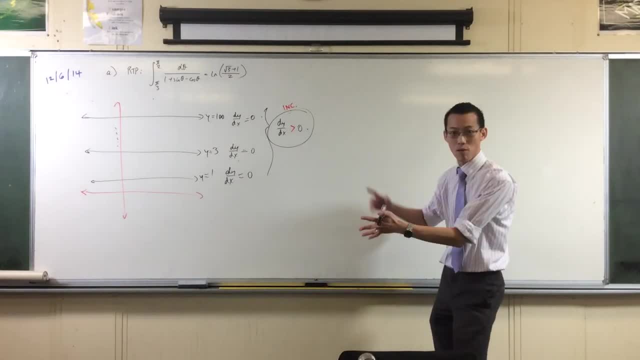 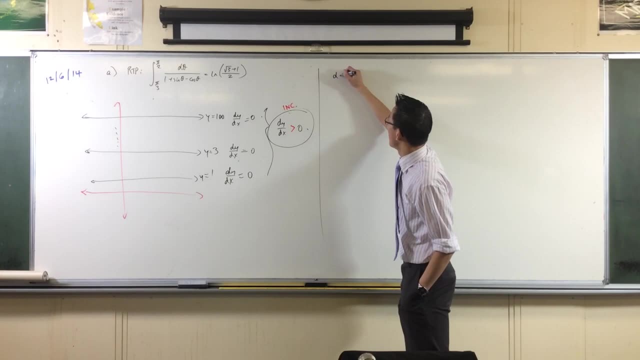 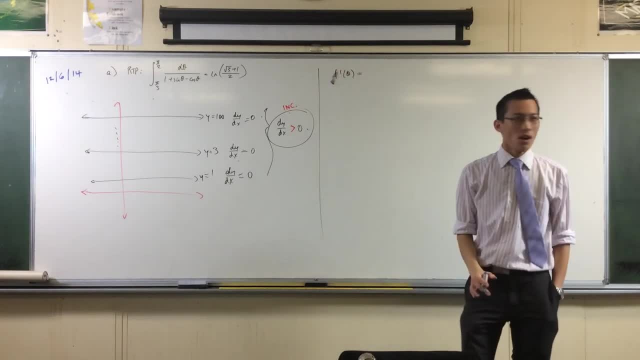 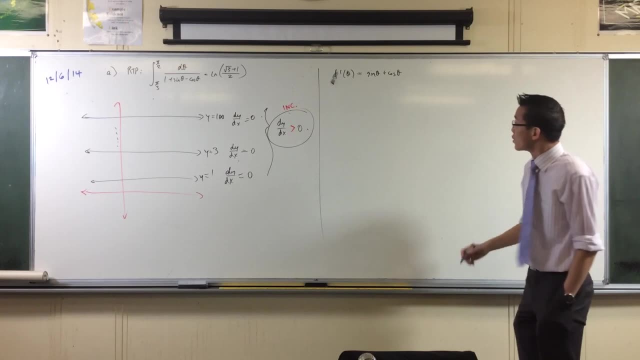 said- you said it all the time- rising to zero plus outside of that, that would be zero, right? Then you said an especular expression for f theta: all set, all of them, raise to 0.. Then you said: f dash theta, It was sine plus cos, wasn't it Right? So you said: well, 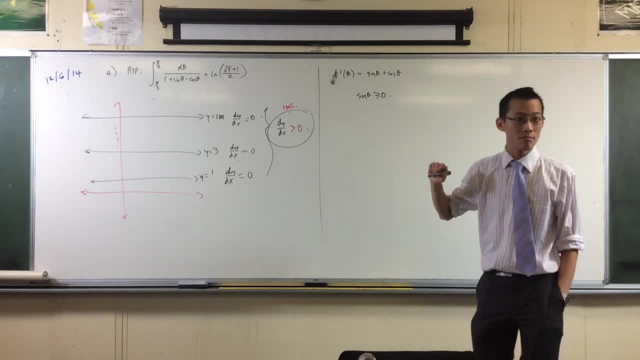 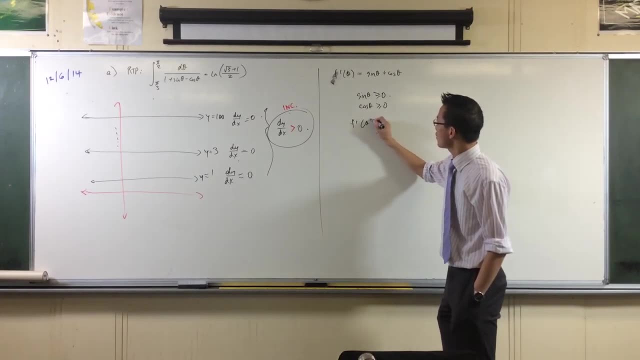 sine theta. well, that's, that's greater than or equal to zero in the domain. right And cos, that's greater than or equal to zero in the domain. So when you add them up, you get this: and that's greater than or equal or equal to zero in the domain, So it's increasing. 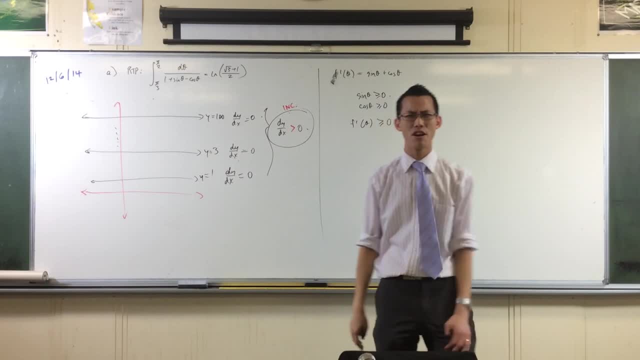 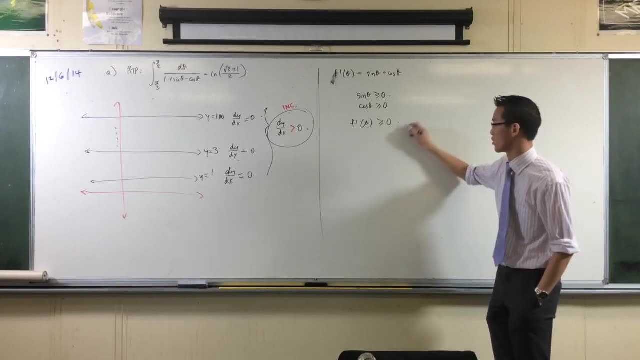 Hurray, just like these guys, we can all be friends, right? No, no, no, no, no, okay. So this is not. this is not qualifying something to be an increasing function. wrong, okay, Others of you saw this. you're like: 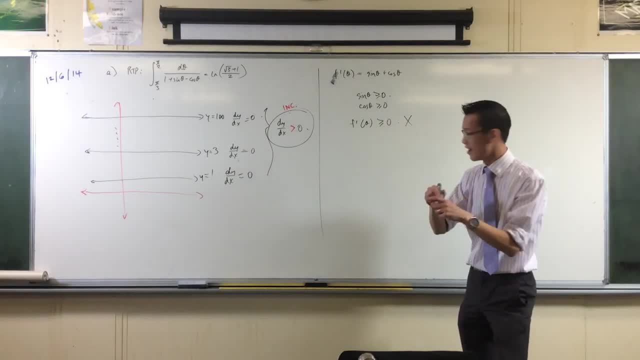 no, I can't. maybe you got to this point. you're like: uh-oh, I can't do that. I need this to be true, right? So you thought mm. I'll backtrack, I can fix this. no problem, white out solves all things. 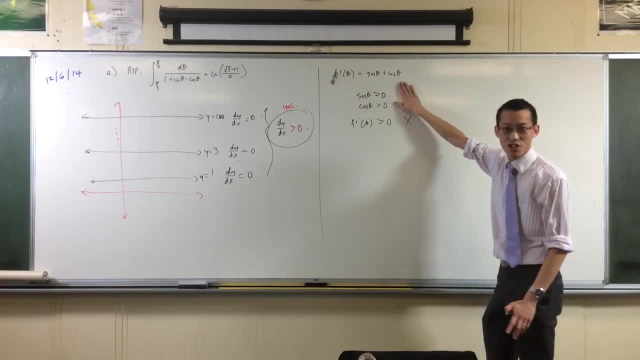 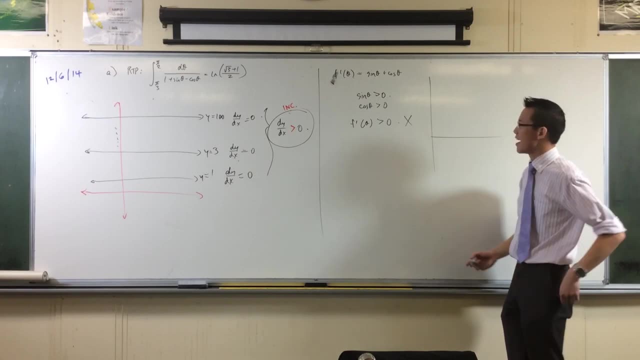 I'll say this, right, I'll say that this is true in the domain. what was it? not to pi on two, Not to pi on two right, Except in not to pi on two sine theta. well, that starts off at zero, bam, okay. 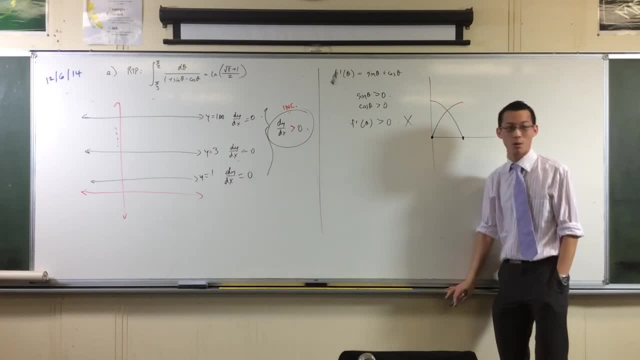 And then cos theta at pi on two, he's equal to zero. Neither of these statements are true, right? So if you tried to fix this by fixing these, that was bad. Still more of you said up here and in back. 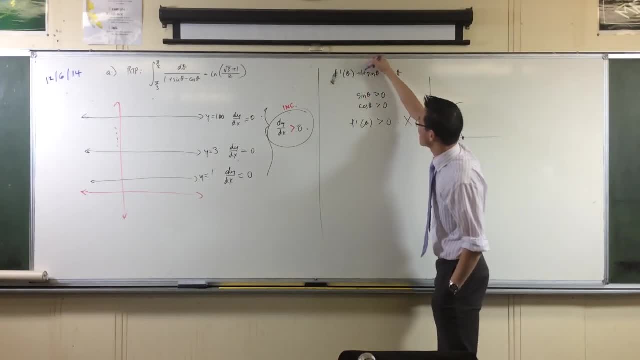 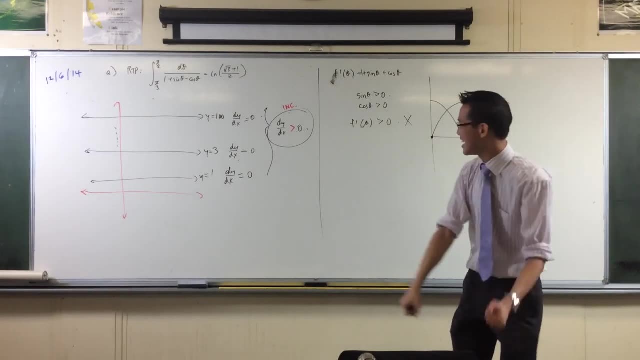 And then, embarrassingly for someone who got a lot of other things right. nah, it's cool. it's cool, The derivative is one plus sine, theta plus, and you add one to all of that, so it's positive. Yes, sweet. 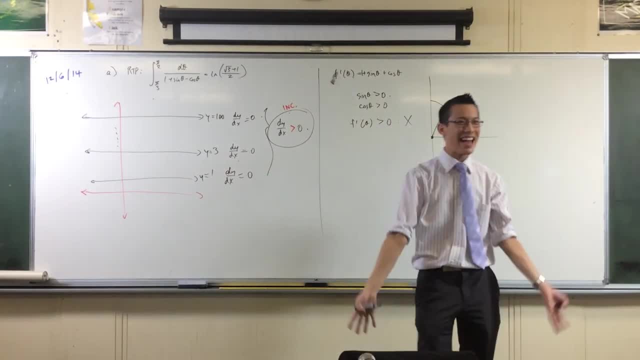 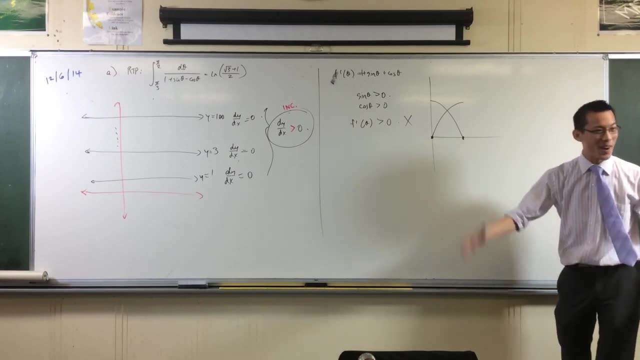 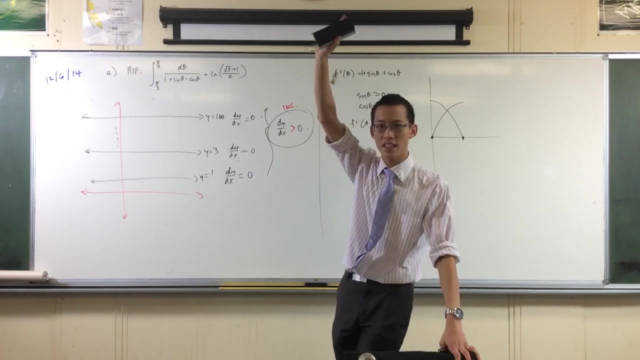 Cos I can differentiate one and get one right. Right, oh, I cried, I cried, I seriously cried. Okay, so now. so, therefore, for actually, who got this right? did anyone get the mark? Now, yeah, I thought so because I knew I might. 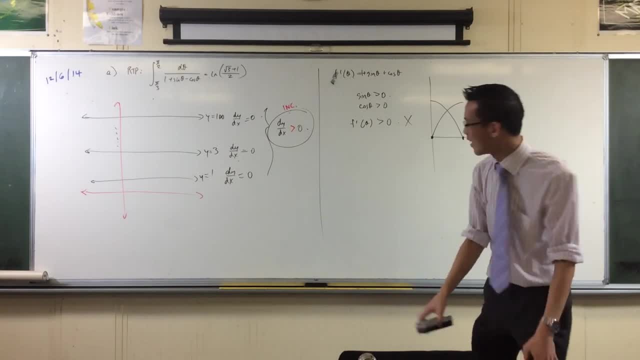 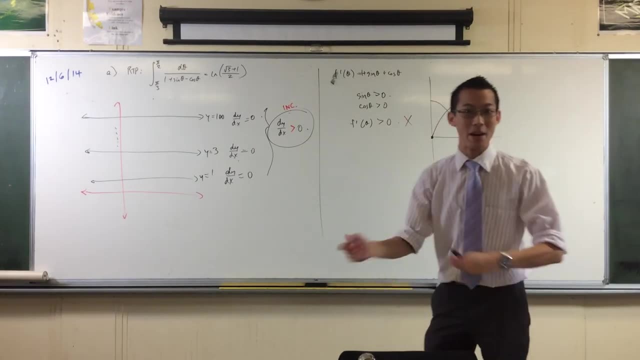 now. so for 24 people who got it wrong and, believe me, tried a lot of different ways, you'll laugh at what was the most simple and elegant way to prove it. Watch Here's sine theta and here's cos theta okay. 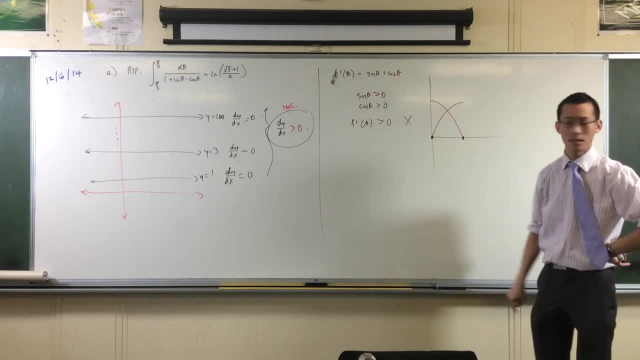 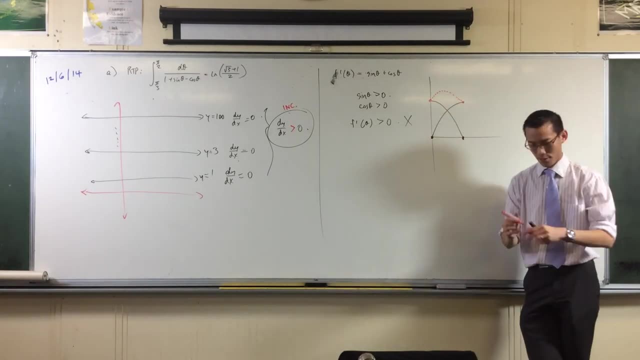 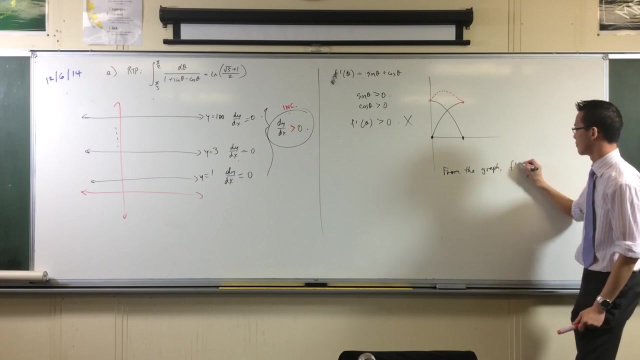 So what does? what does F dash look like Sine theta plus cos theta. Well, it looks like this. So in my solution I wrote this: See you later, suckers. okay, That's all you had to do. 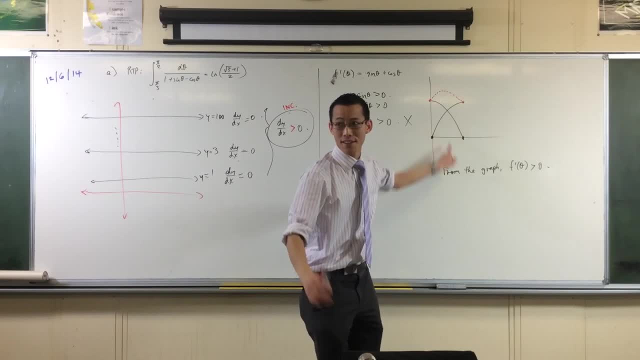 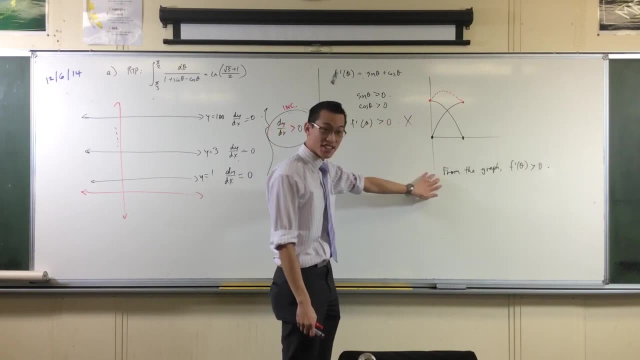 You just had to differentiate graph. it's a simple graph and all of you guys are like, oh, do we have to graph? It takes so long? Yeah, I bet it took a long time, right, And it's such an elegant way to say.